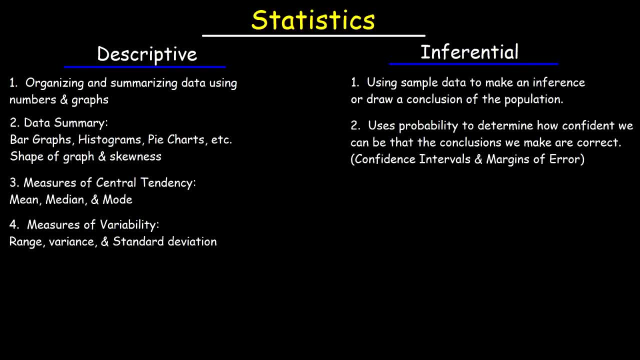 So what is statistics? Statistics is basically the science of collecting, analyzing and interpreting data, even presenting it as well, And statistics can be broken down into two categories: On the left, we have descriptive statistics and on the right, inferential statistics. 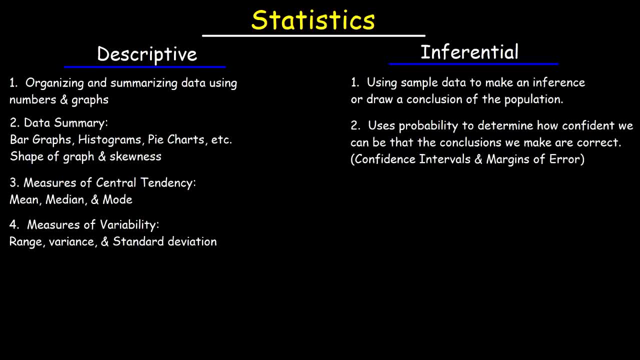 So let's focus on descriptive statistics first, because you're going to learn that first, before you learn inferential statistics. In descriptive statistics, you're basically organizing and summarizing data using numbers and graphs. For instance, you could summarize your data using a bar graph which looks like this: 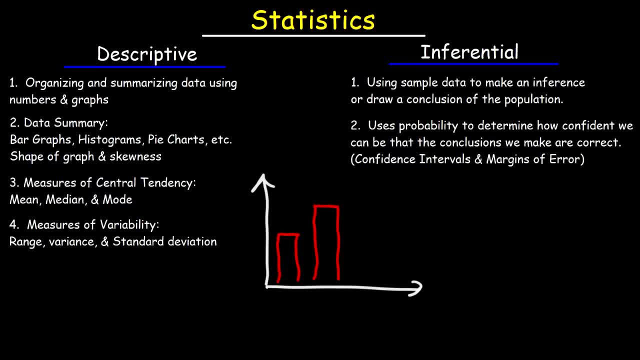 Many of you have seen this in middle school or high school. You could even organize your data into a histogram. A histogram looks like a bar graph, but the bars are basically attached to each other. So that's the difference between a histogram and a bar graph. 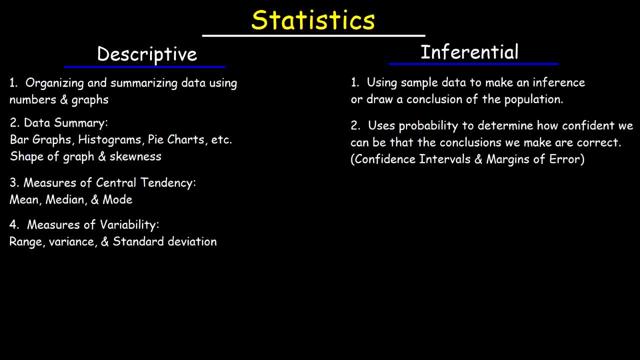 You can also organize your data into a pie chart, And this is very useful if you want to break it down into categories based on percentages. Now, this is very useful if you want to organize your data into a pie chart. there's other graphs too. you have a. you can organize it using a line graph. you 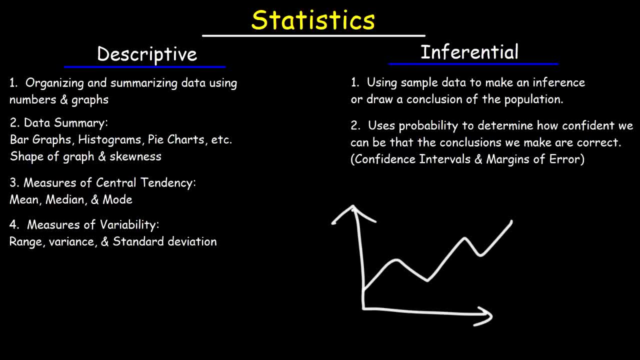 can also use tables to organize your data. you could use a frequency table, a frequency distribution table, and there's a lot of different ways of organizing it, and so that falls under descriptive statistics. you can also describe the shape of the graph, for instance, do we have? is the data symmetrical or is it? 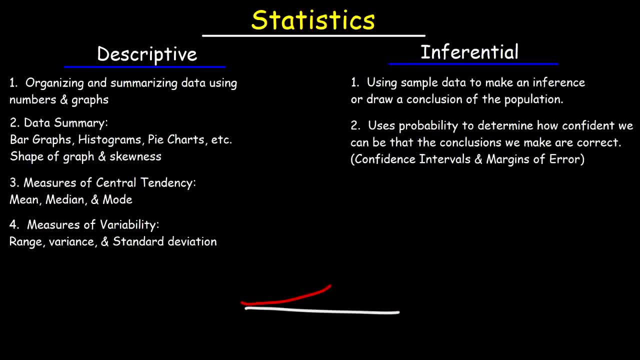 skewed to the right, or is the data skewed to the left so that all falls under descriptive statistics? now we can also describe our data using numbers, so, for instance, under measures of central tenancy, or we have things like the mean, the median and the mode. now there's two types of 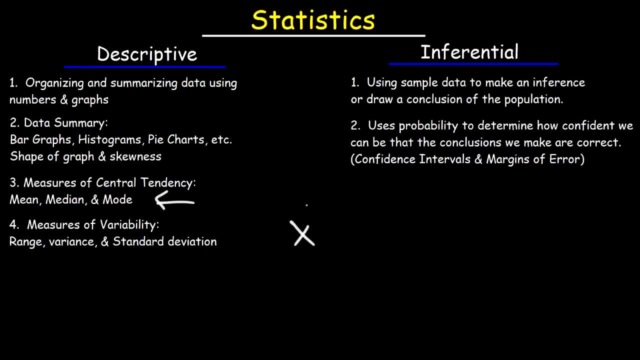 means that you want to be familiar with. the first one is the sample mean, which is basically a sum of your sample data divided by the number of data items in your sample. the second is the population mean, which is also the sum divided by the number of data items in the population. 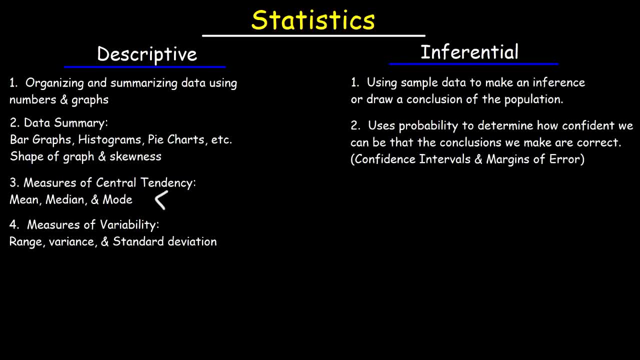 and the mean is basically the average. the median is the middle number of a data set and the mode is basically the number that occurs most frequently. so that's another way you could describe your data. using those types of numbers. you can also describe it in terms of a range variance and standard deviation. 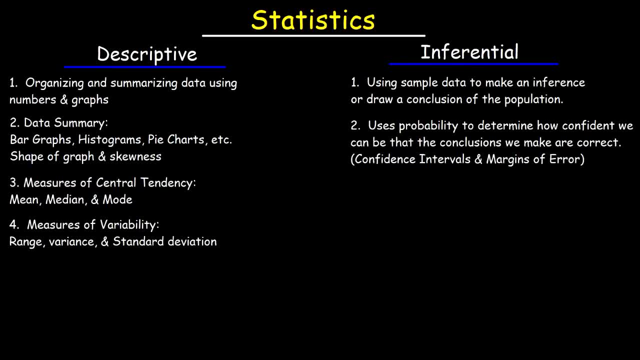 now let's move on to inferential statistics. so in this branch of statistics, that's when we take our sample data and we use it to make an inference or even draw a conclusion of the population- we can even use probability to determine how confident we can be that the conclusions that we make are correct. so 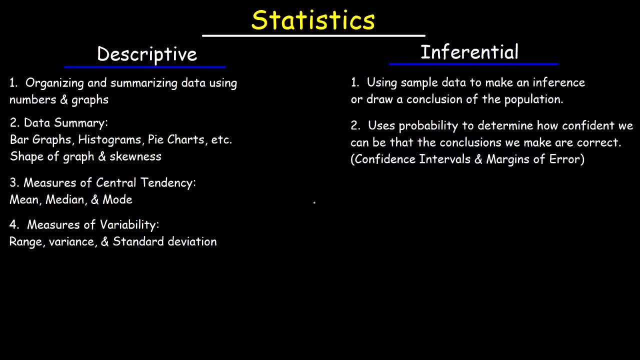 let's use an example to illustrate this. let's say in city XYZ the population is a hundred thousand now and let's say we wish to make a test: how many people in this city like blue cars? how can we find the answer to this question? now it would. 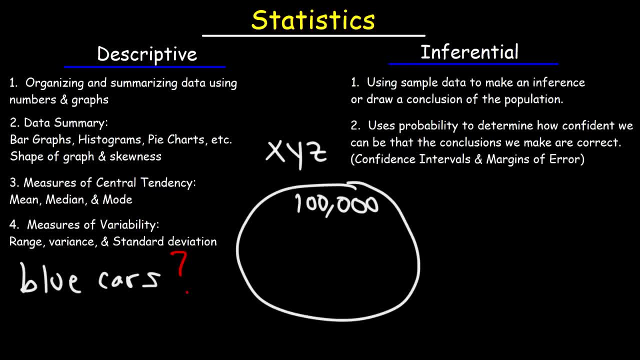 be unreasonable for us to ask every citizen in this city if they like or if they prefer to purchase a blue car, because that means you have to ask one hundred thousand people to make a test. so let's say we wish to make a test for one hundred thousand people, and that's just not practical. so instead, 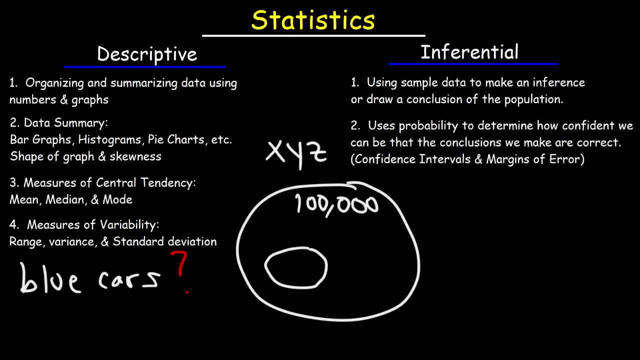 what we could do is take a small sample of the population, let's say a hundred individuals, and ask them: hey, do you prefer to drive a blue car or do you prefer to drive a red car? and see who say yes. now let's say, if 20 out of the 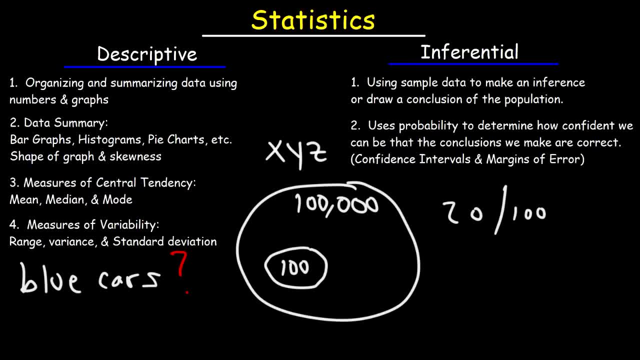 100 people in our sample says yes. so that means that 20 percent of people prefer blue cards. this is based on our sample. that's our sample data. so that would fall under the realm of, would you say, descriptive or inferential statistics. which one now? this is basically a fact. 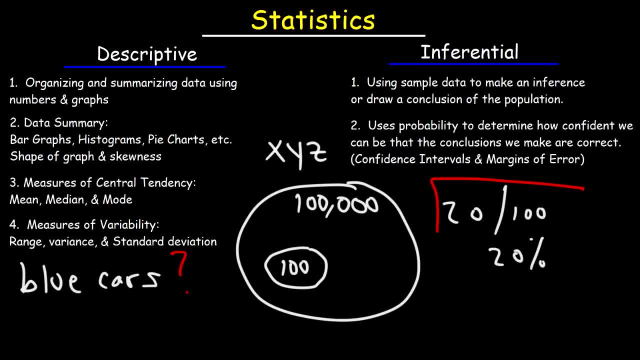 we're presenting data, so 20 people out of a hundred say they like blue cars, so that would be descriptive. now we can use that information to draw a conclusion about the population. we can say that twenty percent of the entire population may be within a two percent margin of error, like blue cars in this. 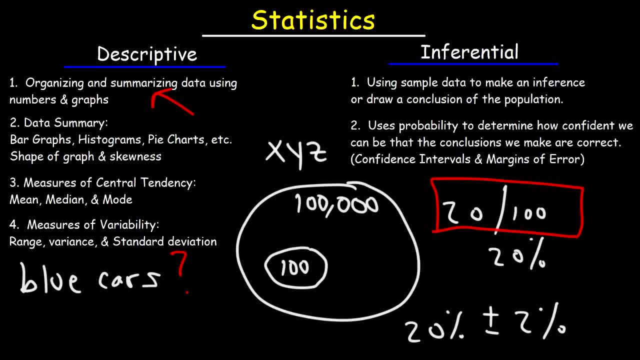 case, because we're making an inference or withdrawing a conclusion that will fall under inferential statistics. now there's something known as confidence intervals, which also falls under inferential statistics. so we could say that we are ninety-five percent certain or ninety-five percent confident that twenty percent of the individuals living in city XYZ prefer to. 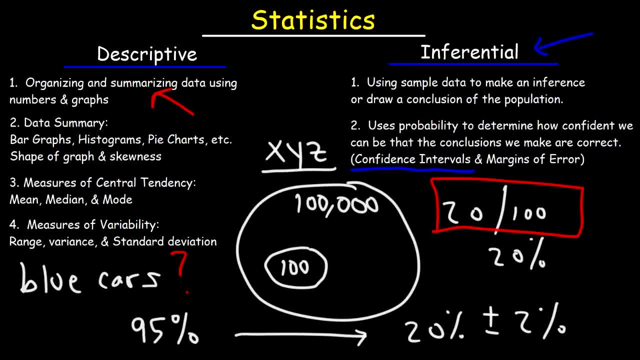 drive blue cars within a two percent margin of error. now we can increase our confidence and get a better picture of the population data and how they like blue cars if we increase our sample size. so let's say we increase it to a thousand instead of 100. so if we ask a 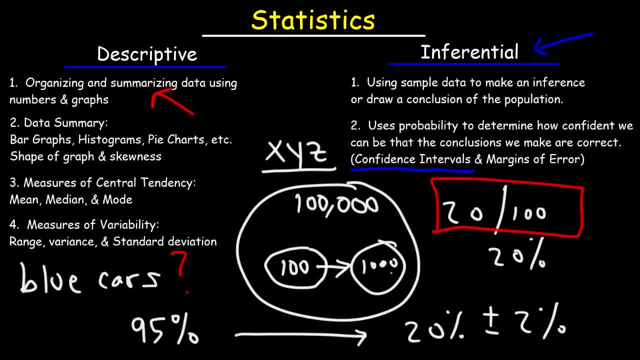 thousand people do. they like blue cars. and let's see, the data is now different. let's say, 21 percent says yes to it within a one percent margin of error. so this value is going to be a better reflection of the population in response to their preference for blue cars, because our sample 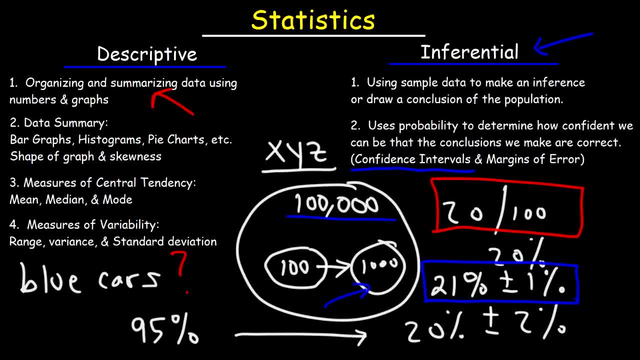 size is bigger. so now we can say that 21% of the population prefer blue cars within the 1% margin of error. so by increasing the sample size you can make a better prediction of the population and their preference for blue cars. and so that's a basic intro between descriptive statistics and inferential. 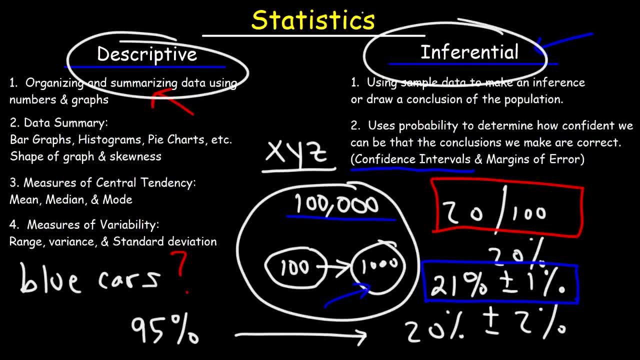 statistics. so hopefully this video gave you a better understanding of these two topics. so that's all I got. thanks for watching. 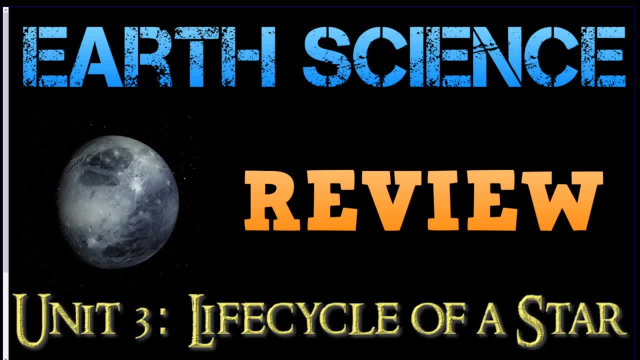 Hi everyone and welcome to the next episode of the Earth Science Review series. This is going to be focusing on Unit 3, Astronomy with the life cycle of a star. So here we go. A little bit of background before we start the practice questions today. 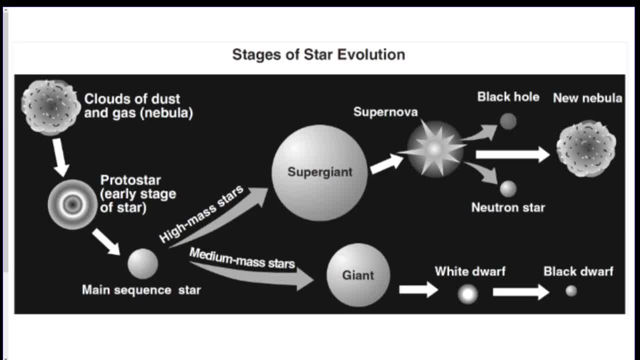 So the first thing we want to highlight today is the stages of the evolution of a star. So the idea is: in this picture, as you can see, all stars start out as a cloud of dust and gas, and this is called a nebula. 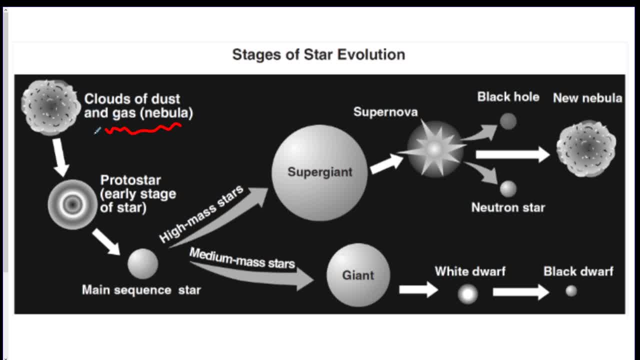 So eventually the nebula gas contracts by gravity and the gravity makes all the dust come together and you get a protostar right here, which is like the early stage or the embryo of a star, essentially. And eventually, when it gets hot enough and there's enough pressure, this process called nucleotide. 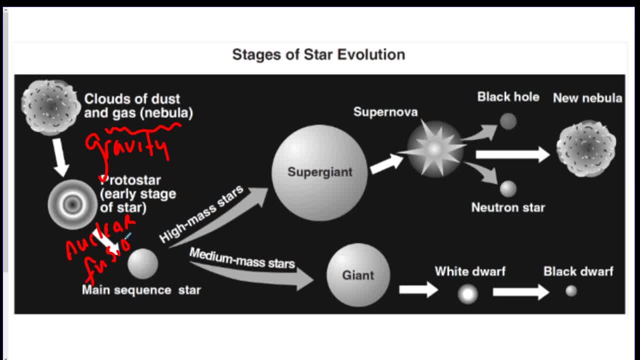 So the moment that nuclear fusion starts to occur, and the moment that nuclear fusion starts it produces heat and light, which is fusing the hydrogen atoms into helium in the center of the star and the star starts to shine. So you need the fusion to start occurring before you get your main sequence, star. 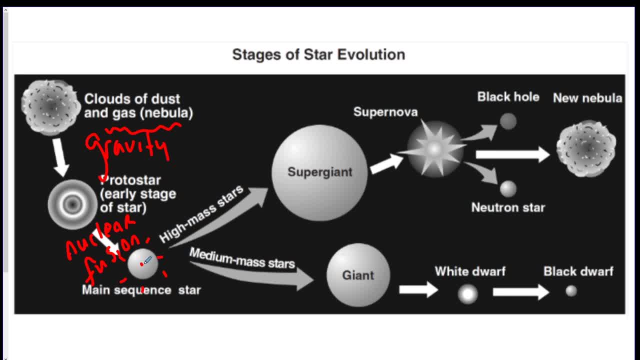 Now all stars end up becoming main sequence stars. Depending on the size or mass of the star is going to depend on which life cycle they go down. So, as you can see, we're going to start with the medium mass stars, so this could be medium to low mass stars. 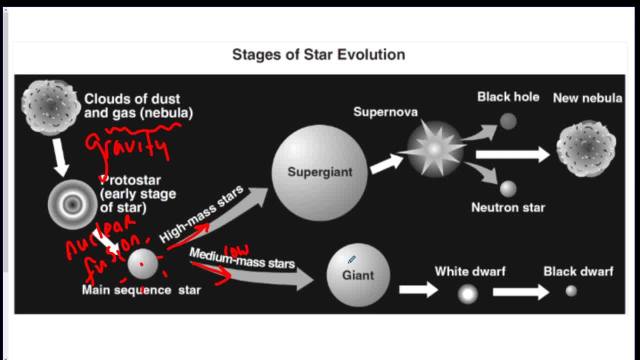 It's going to turn into a giant. Now, the color of the giant depends on the temperature of the star, which we'll get to eventually, but the red are generally cooler temperatures than a blue star might be. This is going to be the path that our sun takes, because our sun is an average size star.